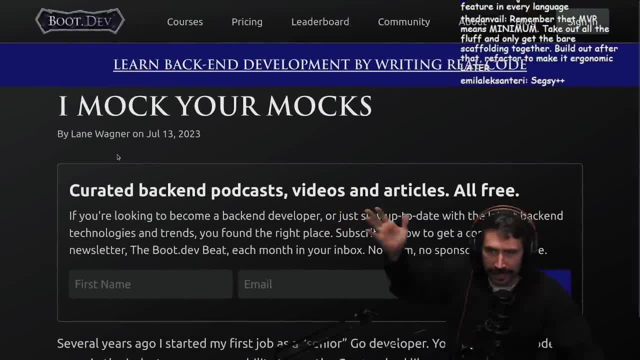 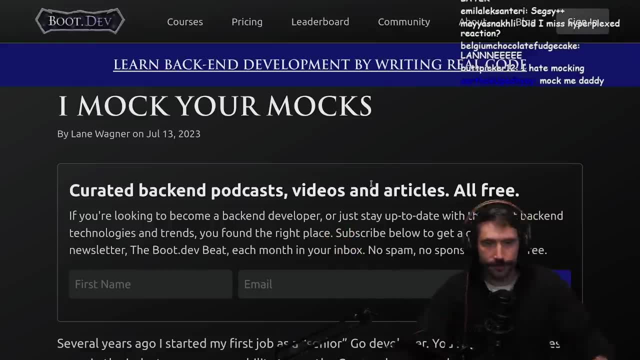 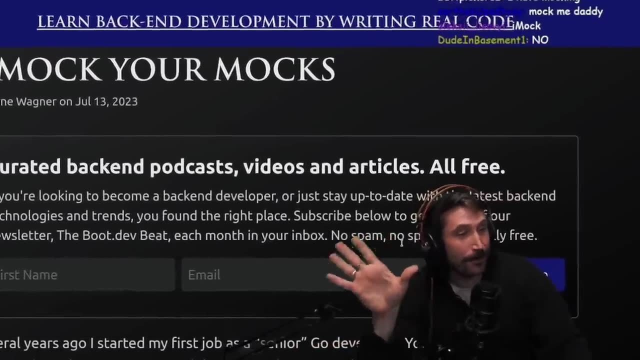 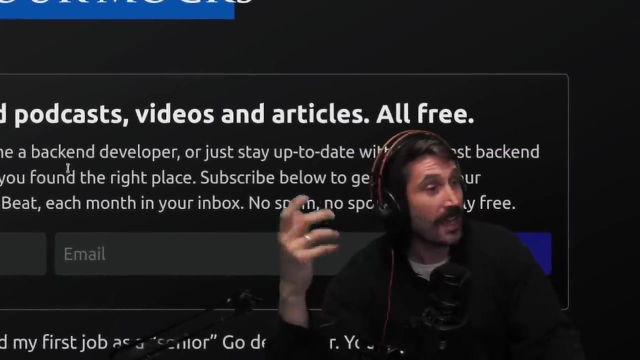 Alright, first off, I mock your mocks. This is by Lane. If you don't know, Lane bootdev Great stuff: Learn back-end development by writing real code. So it's like a site to learn stuff with. You know what I'm talking about. This is technically a sponsored read. I want to say that right now. okay, But I get the opportunity to say what I want about it and I get to pick the topic, and this is a great topic. This is perfectly what I want to talk about, because I have many, many strong, strong feelings about mocks. Yeah, sponsored Hashtag ad. I got to say it up front because I want to be an honest individual, okay. 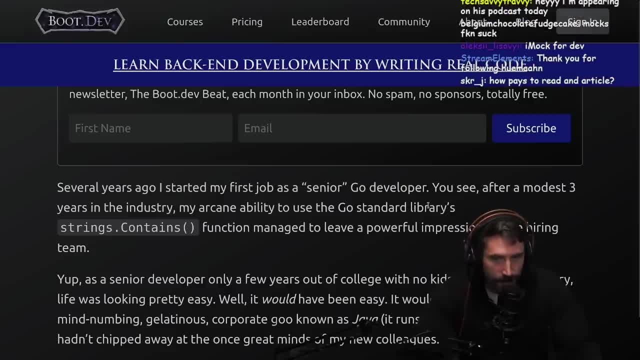 Okay, Several years ago I started my first job as a senior Go developer. A lot of scare quotes going on here. You see, after a modest three years in the industry, my arcane ability to use Go's standard library string contains function managed to leave a powerful impression on the hiring team. 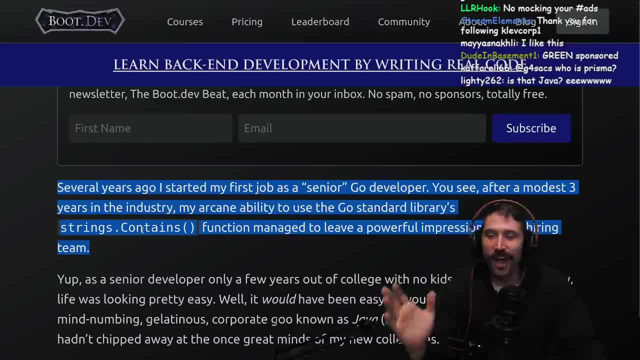 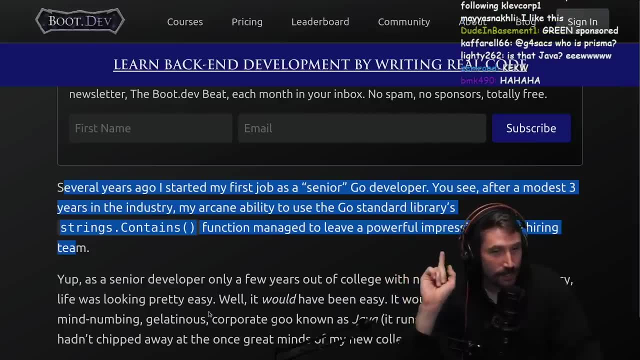 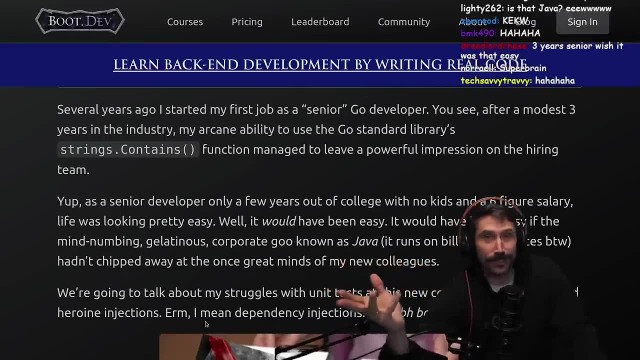 Yes, Yes, Okay. so first off, he may not realize what he's saying, but there is something that's really good here, which is: know your language, you dummies. You walk into an interview, you can just magic them with some really simple stuff that's just available because that's what's available in your language. 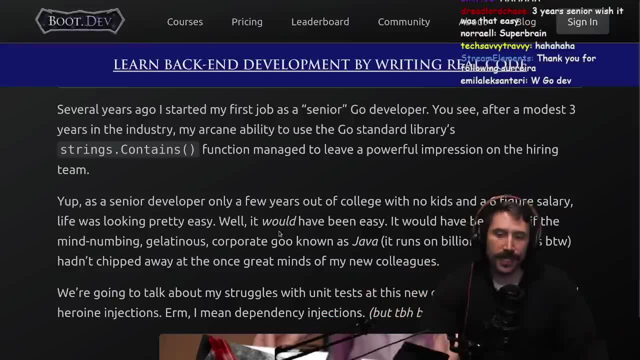 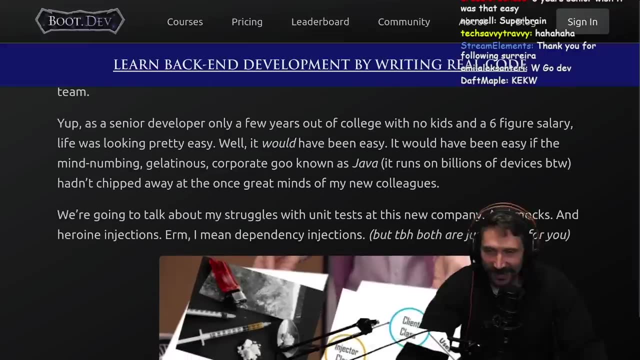 Just know the things. Yep, as a senior developer, only a few years out of college, with no kids and a six-figure salary, life was looking pretty easy. Well, it would have been easy. It would have been easy if the mind-numbing, gelatinous corporation goo known as Java. it runs on billions of devices, by the way. 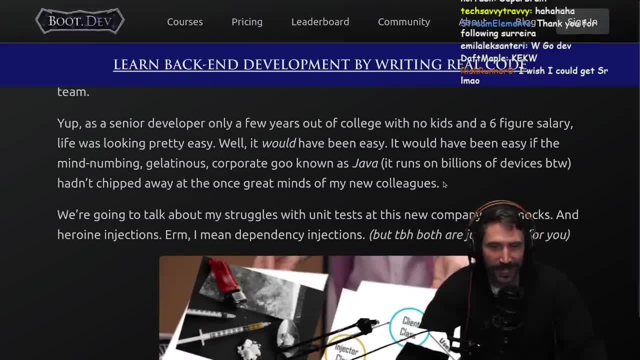 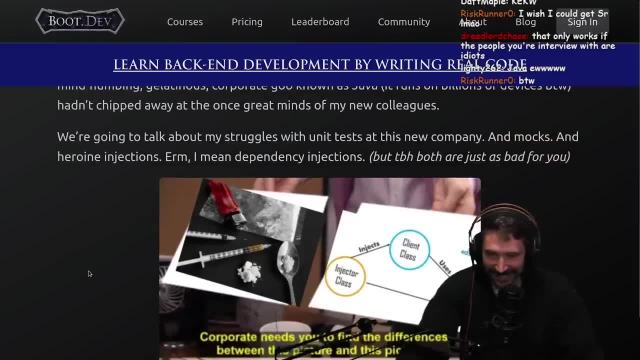 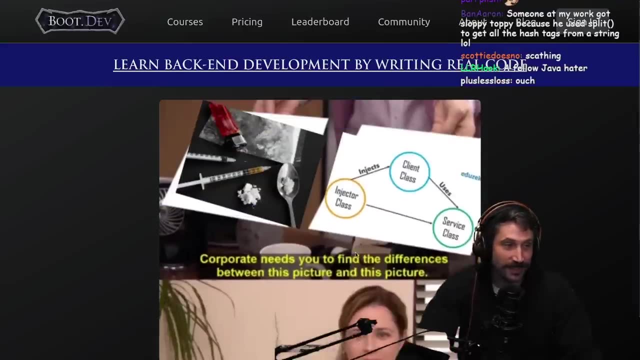 hadn't chipped away at the once great minds of my new colleagues, Java, by the way. Oh no, Oh no, Corporate needs you to find the difference. Okay, that's actually a really good meme. This is a really good meme. 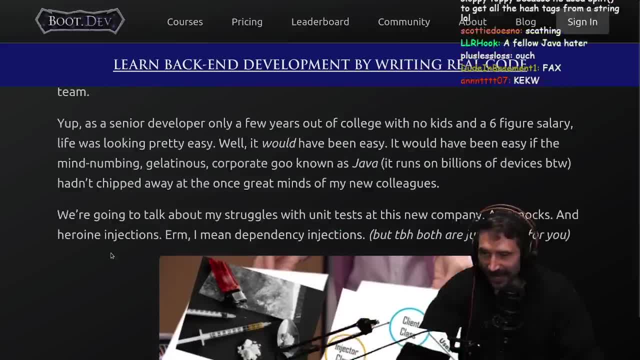 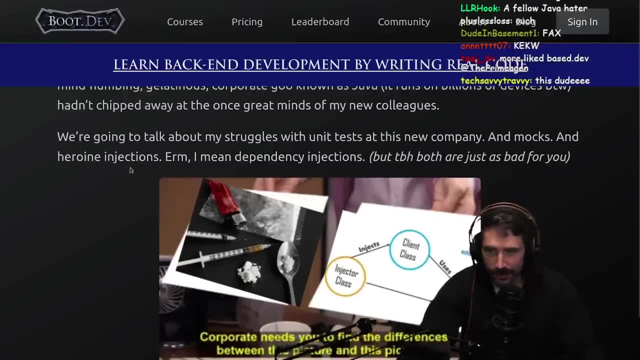 Hard drugs, free basic. Actually, that's just straight banging heroin. We're talking about my struggles with unit tests at this new company and mocks and heroin injection- I mean dependency injection. To be honest, they're both just as bad for you. 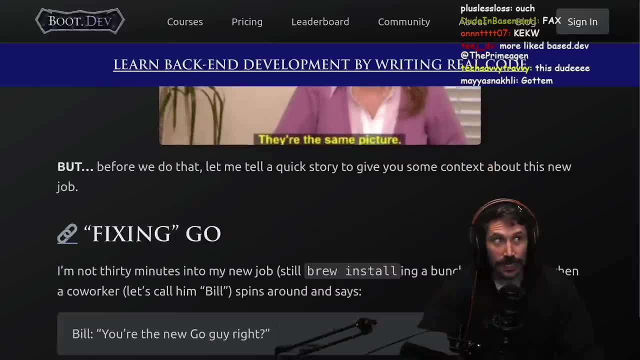 I am on the same team. In general, I am a huge, huge advocate for never mocking. I'm on team never mock, Okay, Okay, Never mocker right here, Okay. Before we do that, let me tell you a quick story to give you some context on this new job. 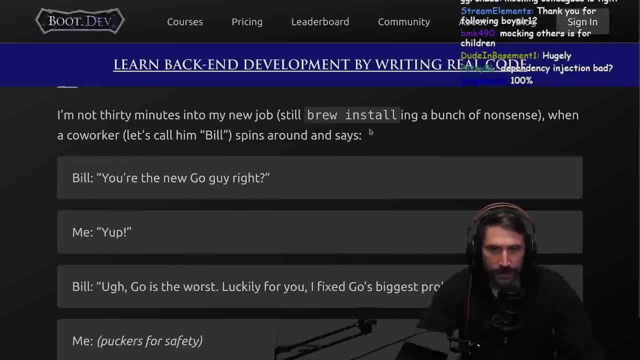 Fix and go. I'm not, 30 minutes into my new job, still homebrew, installing a bunch of nonsense. when a coworker- let's call him Bill Bill, You know it's no Tom, I'll tell you that much. There's no Tom right now. 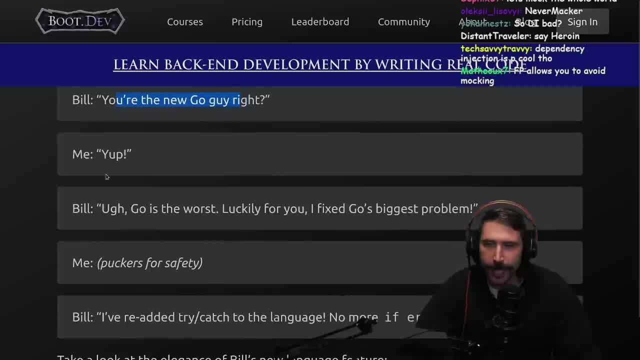 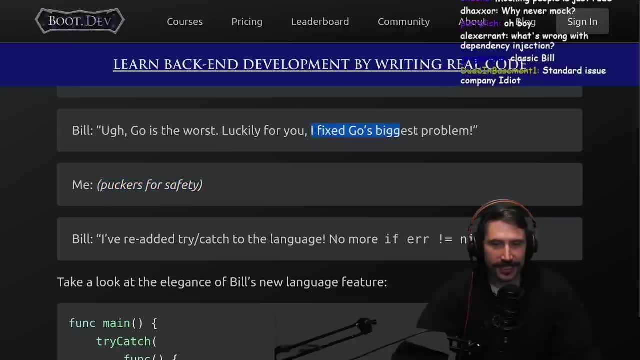 Spins around and says: hey, you're the new go guy, right? Yeah, Go is the worst. Luckily for you, I fixed Go's biggest problem. If someone actually says this like, hey, I fixed TypeScript's biggest problem, I know immediately that whatever they fixed is probably worse than the thing itself. 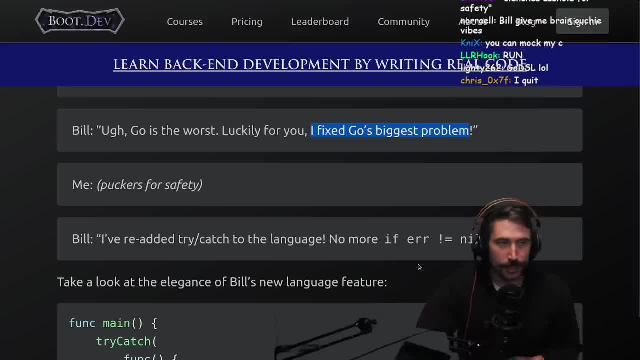 I hate to say it, but you're not making things better. Okay, You're not doing a good job. Bill's the genius in this story. I smell a Tom. I smell a Tom. I've re added: Try catch the language. 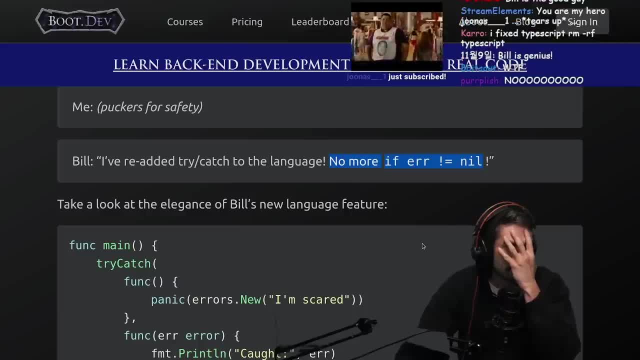 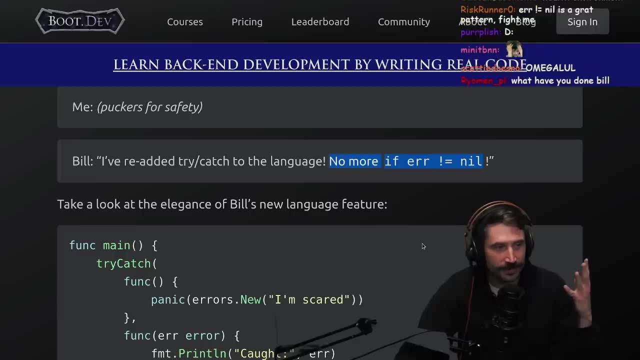 No more If error equals nil, Welcome to Costco. They say. if your hand is bigger than your head, you're likely to get cancer later in life. By the way, that was a joke from the 90s to get kids to put their hands on their faces, and then you hit their hand and so that they hit their own face. 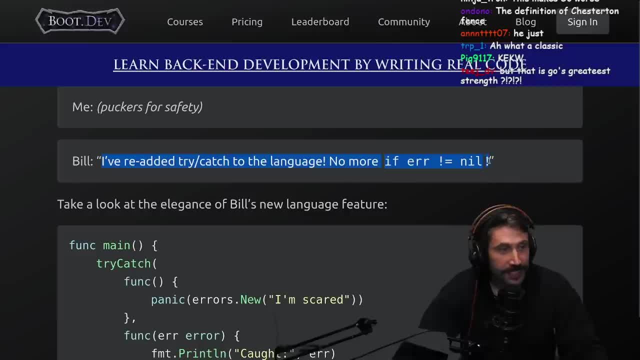 Okay, That's pretty much what you're doing right here. This is the exact same joke, Except for it's in code and you don't get to hit your face once. You get to do it every single time you program This is did that all the time? 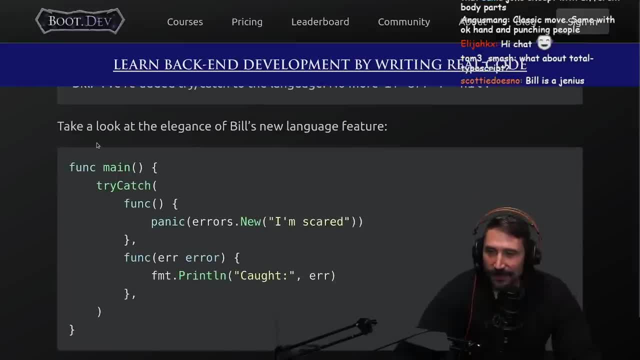 Everyone did it. It was a great joke. It worked every time. Take a look at the elegance of Bill's new feature: Funked- Try catch Funked. Panic Errors- New- I'm scared. Funked Error. 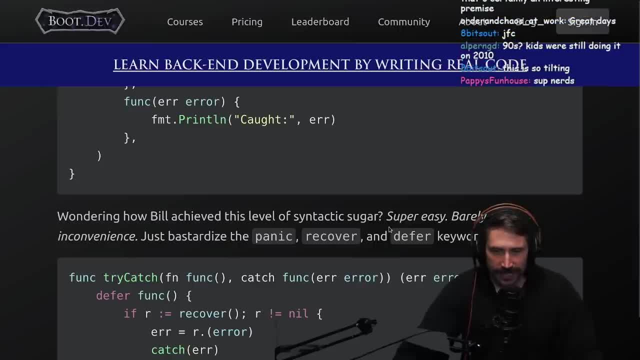 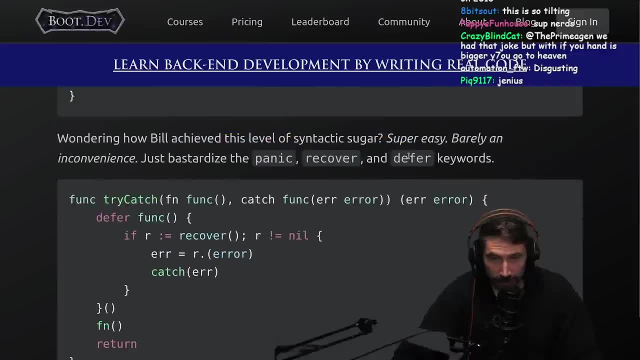 Error Print caught Wondering how Bill achieved this level of syntactic sugar. Super easy, Barely an inconvenience. It just bastardized the panic. recover and defer keywords: Oh gosh, The defer. Oh no, Oh no. 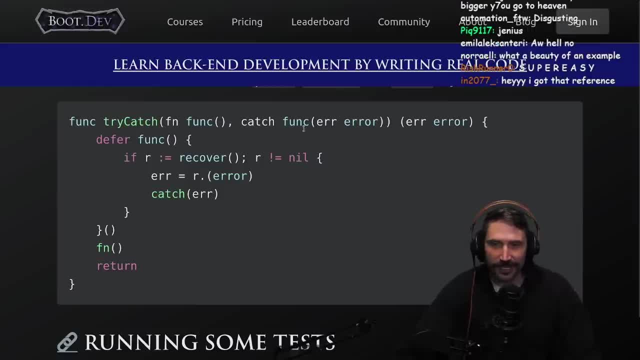 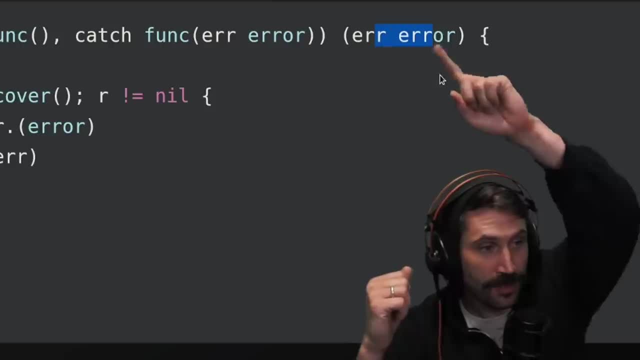 Try, catch, funk, funk, catch, funk, error, error, This, Oh my goodness, That's even a named. I hate naked returns. This is the devil. By the way, this is actually. this is the biggest crime against humanity. 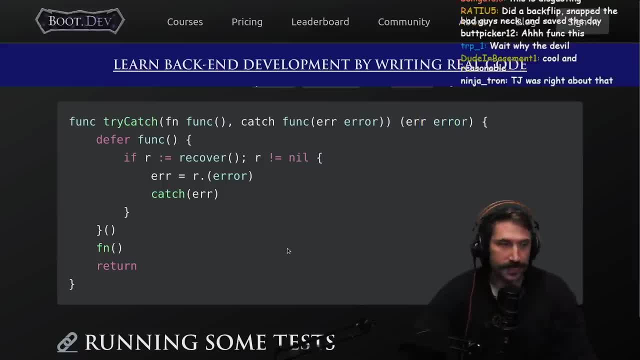 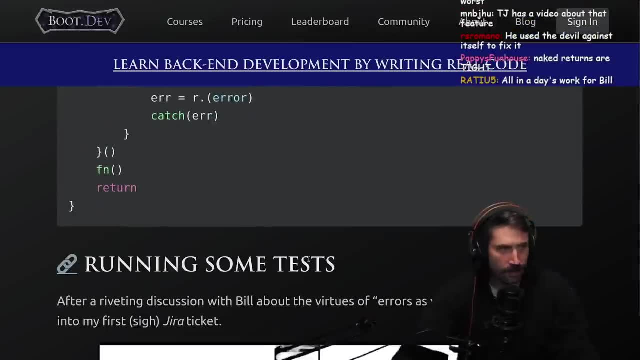 This is Go's worst feature. Naked returns are disgusting. TJ was right about it, Absolutely TJ was right about it, because you have no clue what the F is going on. Naked returns are the devil, are tight. No, they're not. 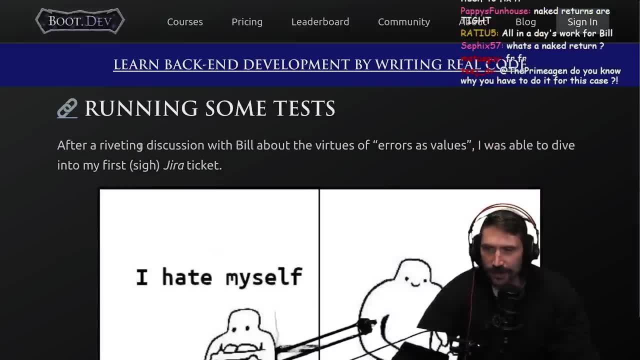 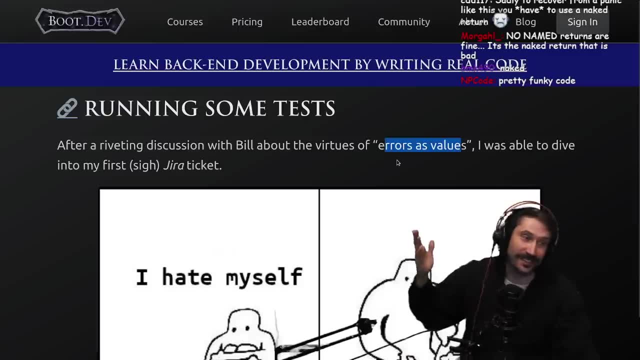 They're tight with the devil. Okay, Running some tests. after a riveting discussion with Bill about the virtues of errors as values- I mean I'm on camp errors as values any day of the week- I was able to dive into my first Jira ticket. 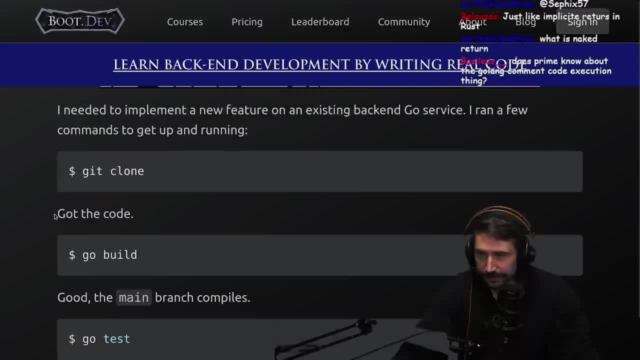 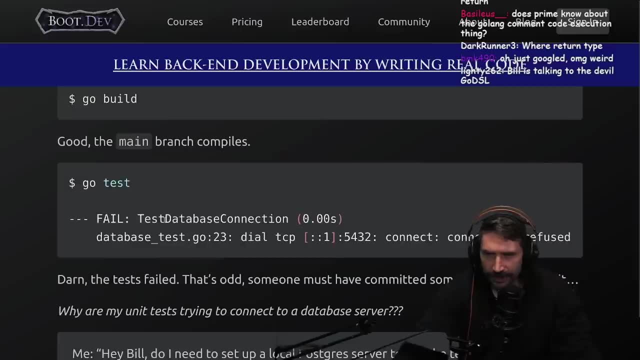 This is correct. This is 100% correct. I need to implement a new feature on an existing backend Go service. I ran a few commands to get going: Get clone Go, build Go test. Failed database connection: Connection refused- Awesome. 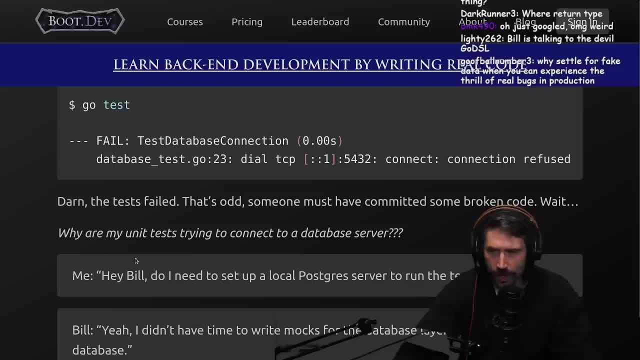 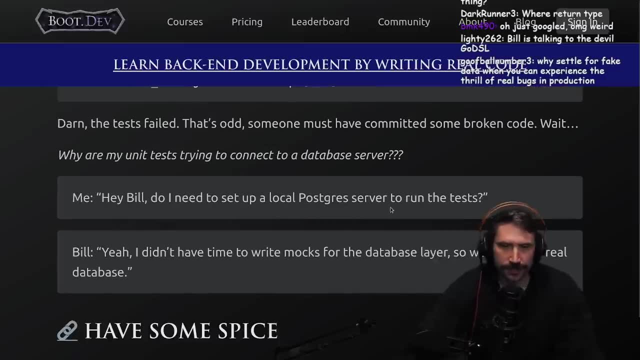 Darn, These tests failed. That's odd. Someone must have committed some broken code. Wait, why are my unit tests trying to connect to a database server? Hey Bill, do I need to set up a local postgree server to run the test? 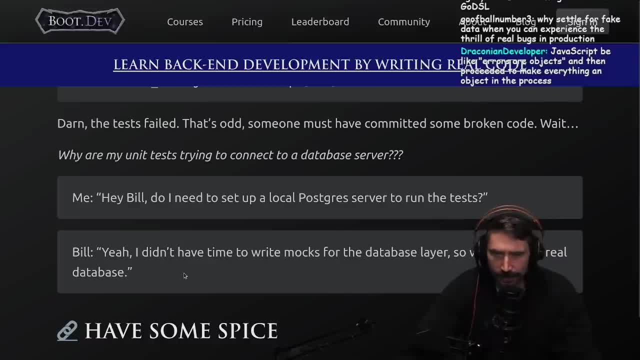 Yeah, I didn't have time to write mocks for the database layer, So we just use the real database. I will. I just want to take a really quick second to say one of the glories of SQL Lite is that you can point to a file even if the file doesn't exist, and it can. 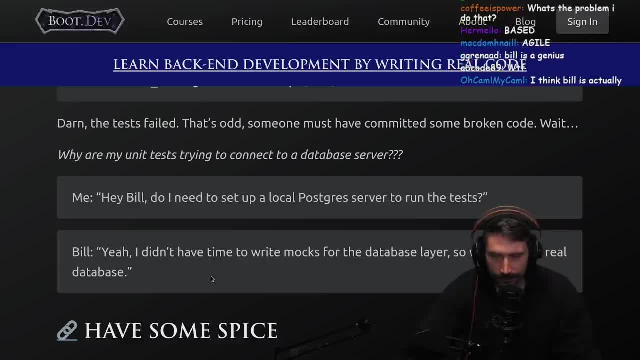 create a database right in that File, and so therefore, for this type of test, if you truly just didn't want to mock anything, you could have a file that just has the database in a specific condition and then just CP the file, put it in a specific location and then run your test on it. 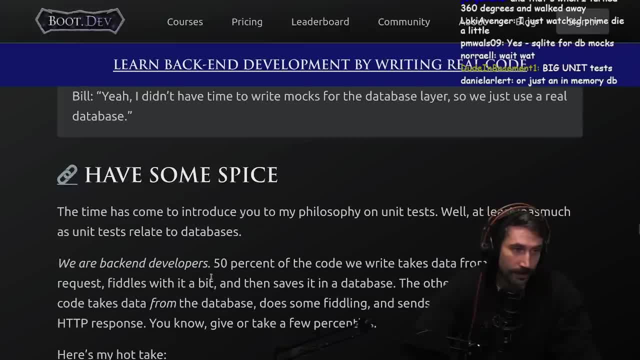 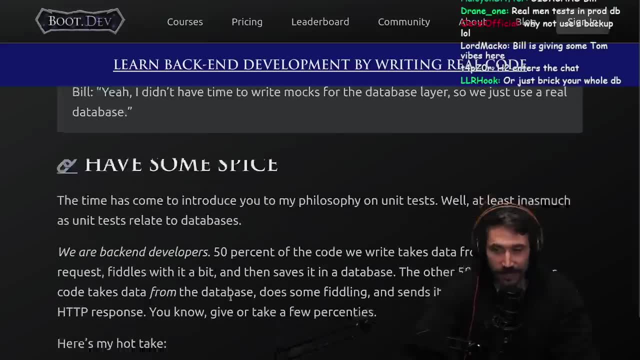 So that is one nice part, But you know what, If you're connecting to a database on a unit test, you done jump the shark. Okay, I just want to let you know that right now your job is in a sunsetting position. 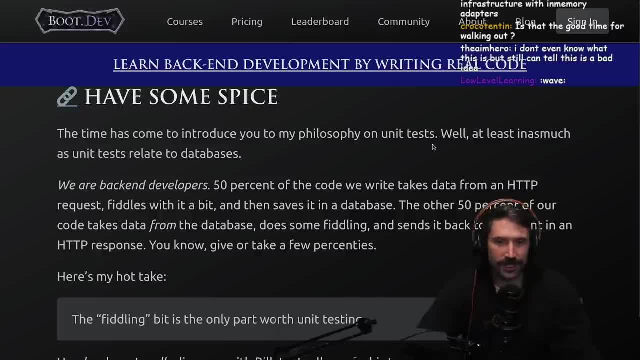 You got to get the hell out of there. The time has come to introduce you to my philosophy on unit test. Well, at least in as much as unit test related to databases, We are back in developers. 50% of the code we write takes data from HTTP requests, fiddles with it a bit. 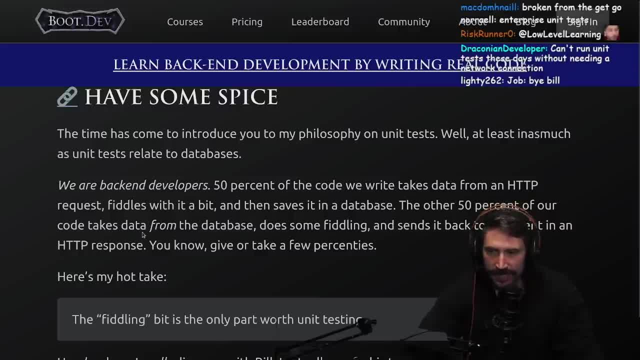 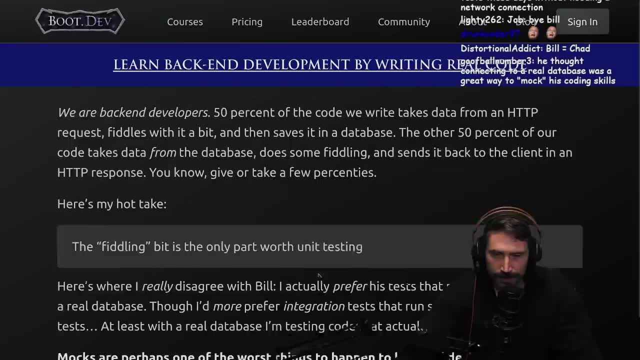 and then saves it to a database. The other 50% of our code takes data from the database, does some fiddling and sends it back to the client in the HTTP response. You know give or take a few percenties. 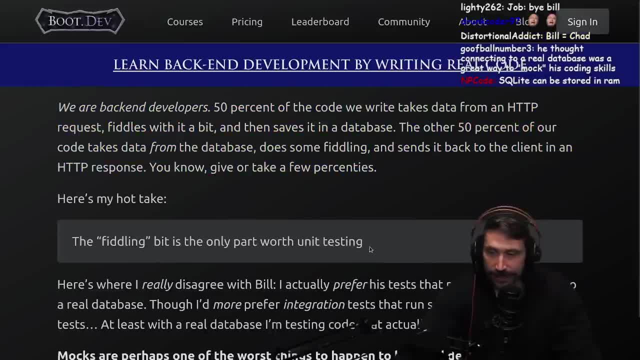 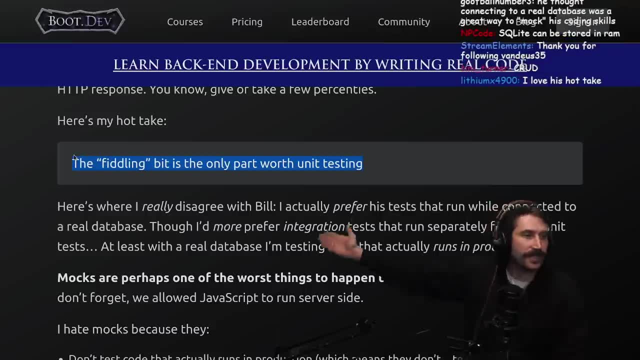 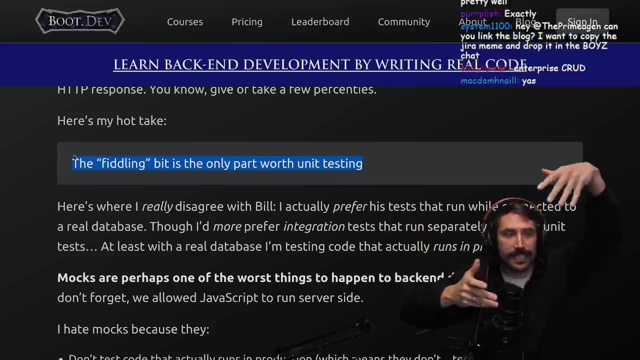 Genuinely fairly well done. Here's my hot take: The fiddling bit is the only part worth unit testing. How many times have I said this? You always have the fiddling part as its own function that takes in the thing you wish to diddle. 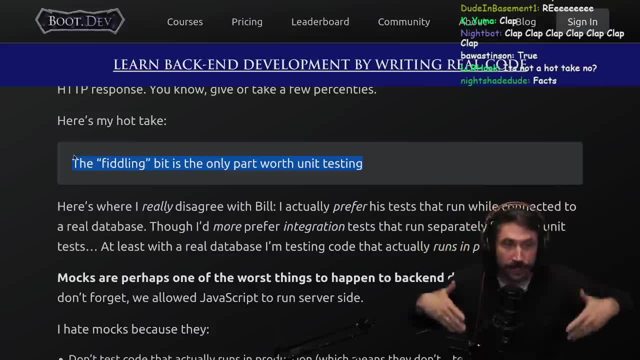 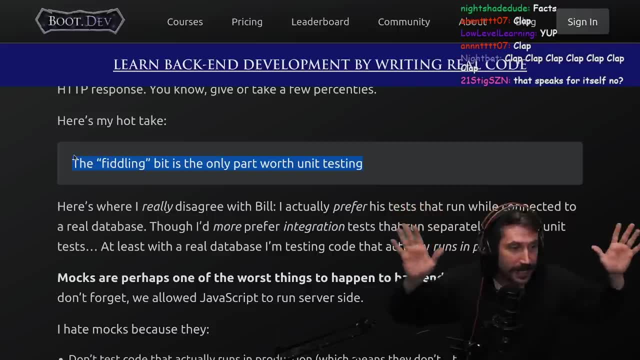 You do the diddling and you return the diddled. Stop having functions that both get data and diddle the data. Okay, It's not worth it. And yes, I'm saying diddle not fiddle because it's funnier. 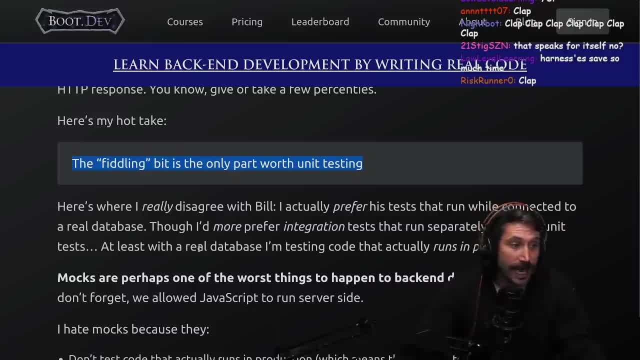 Okay, It is shocking how often people don't do that. Okay, It is shocking that that's not a real thing. My time in seminary was about diddling What. I don't even know why I read that. Here's where I really disagree with Bill. 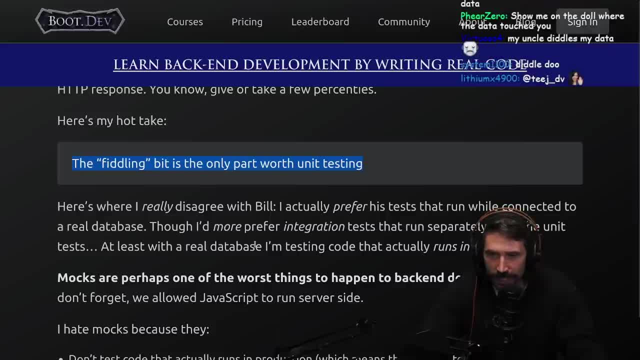 I actually prefer his tests that run while connected to a real database, though I prefer more integration tests that run separately from the unit tests, At least with the real database. I'm testing code that actually runs in production. Mocks are perhaps the worst thing, one of the worst things to happen to back-end development. 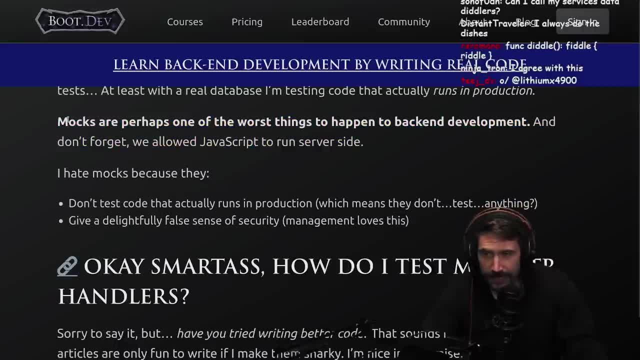 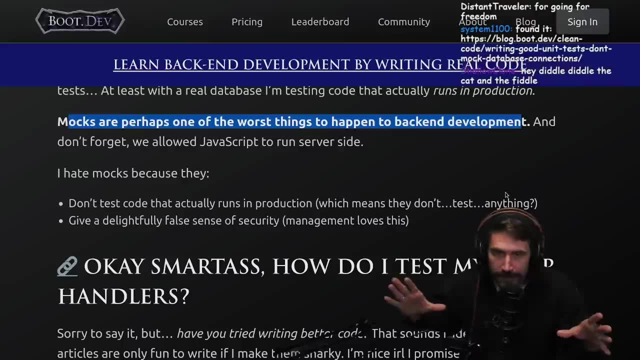 It's actually just the worst thing to happen to all development, not just back-end development, Because here's the problem: It gives you all the power to do integration tests in unit tests, So you end up testing just the stupidest stuff in the universe. 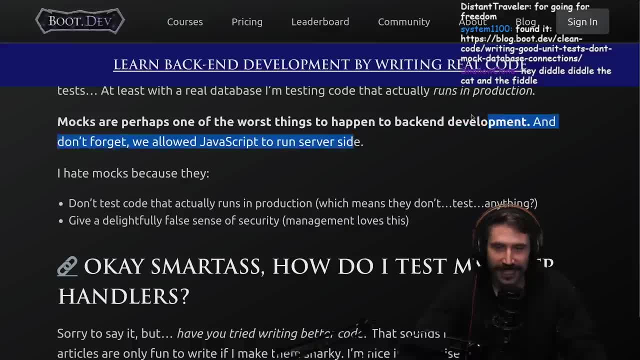 And don't forget, we allow JavaScript to run on the server side. I like Lane. I like Lane. I hate mocks because they don't test code that actually runs in production, which means they don't test anything, Give a delightfully false sense of security. 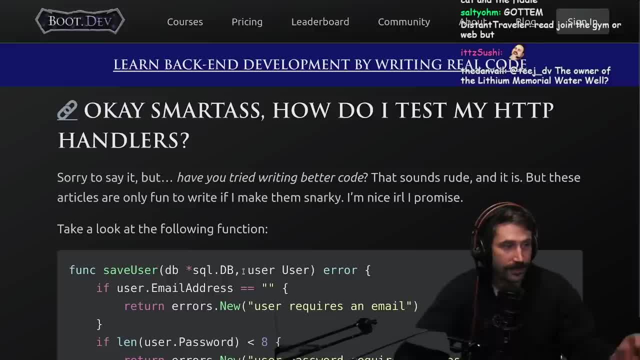 Management loves this. These are all facts. These are all facts. These are all facts. I don't like this song that's playing. It's way too intense. We got to change the song immediately. I am not in love. I am not in love right now. 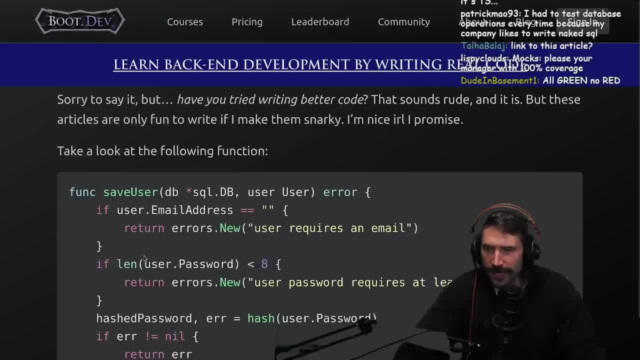 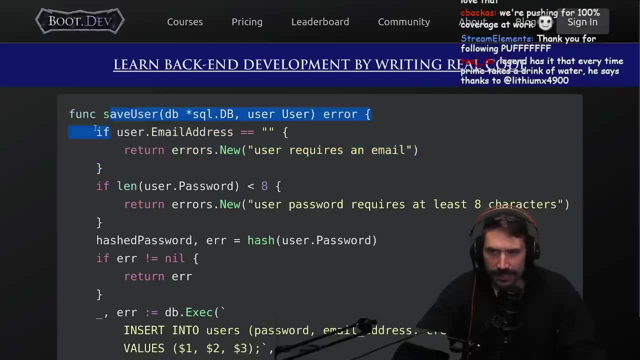 All green, no red, Always green. All right, Take the following function: db squeal user If email address equals null. OK, so I can already tell why you've f'd up. OK, see this line right here. This line should be in a. 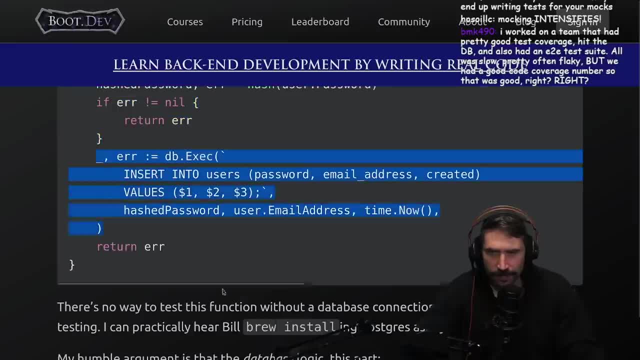 This should all be in a different function. right there, This is the only thing that should be in this function. Right? This is it. This is the only thing that should be in this function. The rest, By the way. look at him. 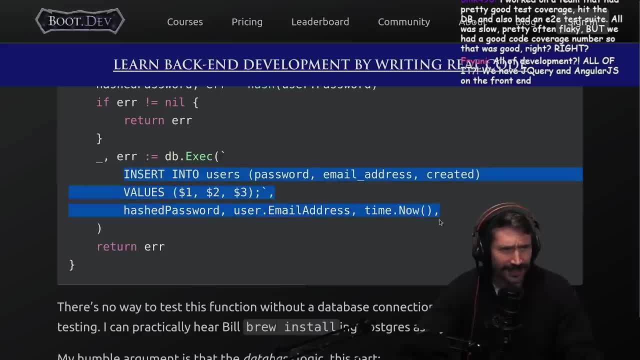 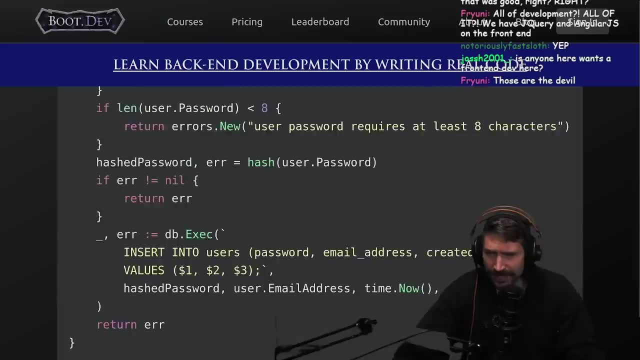 Look at this guy: just raw dog and a squeal. Look at that. Can you believe there's raw dog squeal right now? Like I mean, how would anyone ever raw dog squeal? It's impossible, right. He needs an ORM immediately. 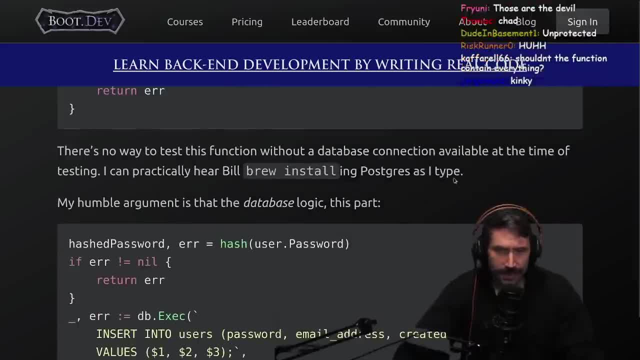 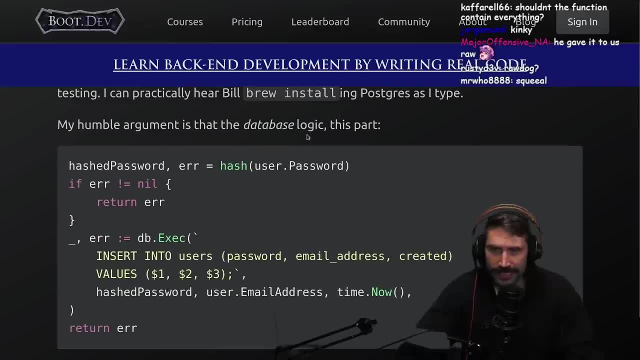 All right, so save user. OK, there's no way to test this function without a database connection available at the time of testing. I can practically hear I can practically hear the whole brew installing Postgres as I type. My humble argument is that the database logic, this part, 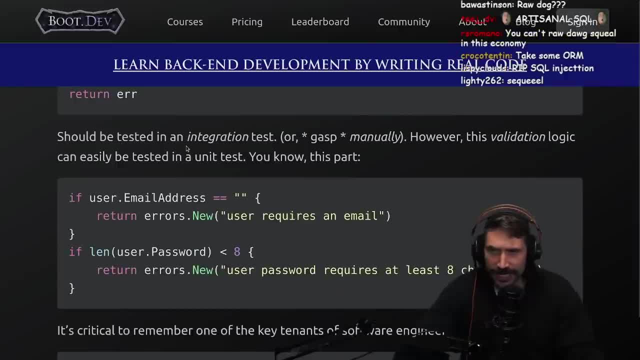 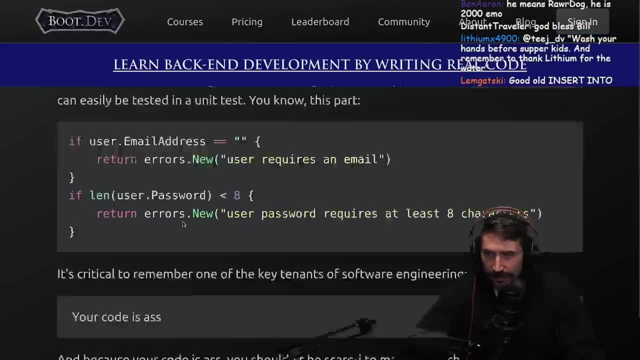 Right Should be tested in an integration test or gasps manually. I'm fine with that. However, this validation logic can easily be tested in a unit. You know, Yep, This part, Yep, absolutely. Me and Lane are like notice, we're on the same page. 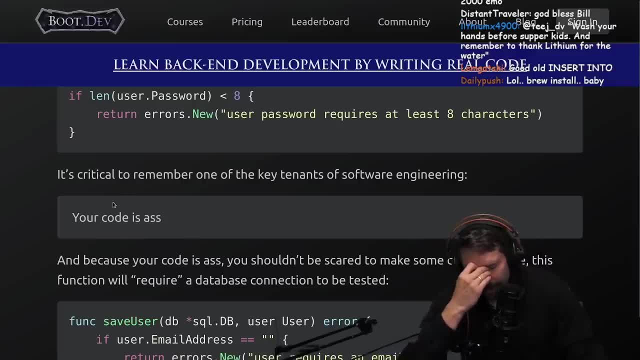 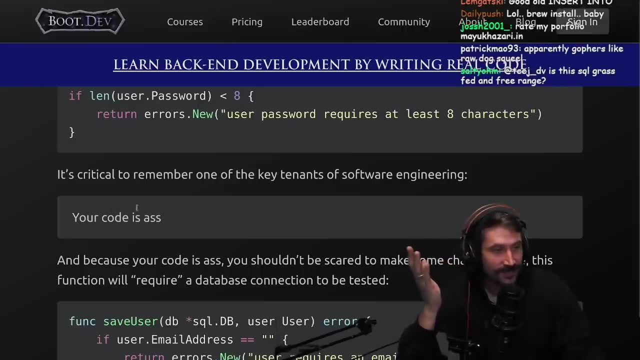 By the way, Lane and I had like an hour long talk, and part of our hour long talk involved us just hating mocks just for like an excessive period of time. So I'm not shocked at all that this this somehow came out as as an article. 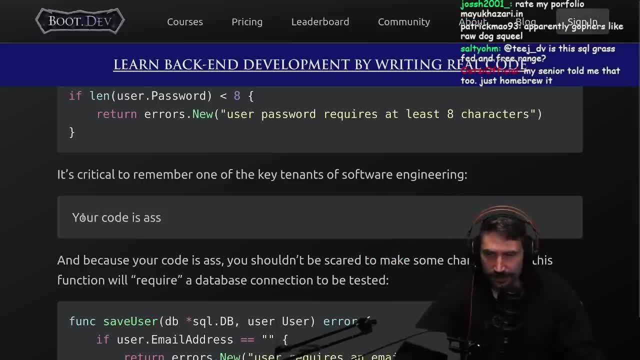 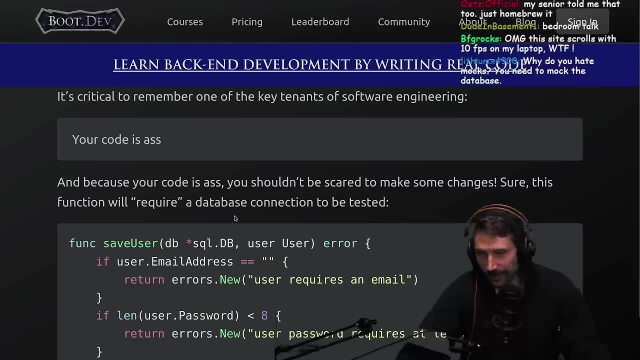 It's critical to remember one of the key tenants of software engineering: Your code is ass, It's facts. And because your code is ass, you shouldn't be scared to make changes. Sure, this function will require a database connection to be tested. 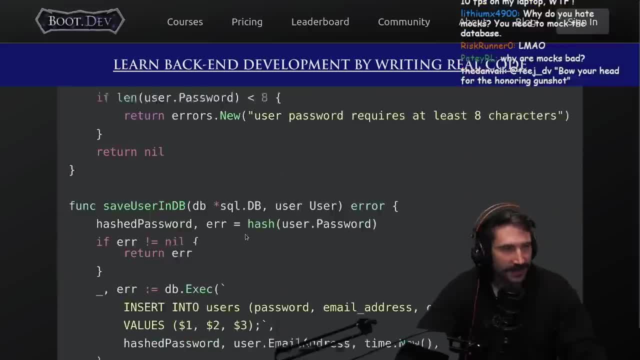 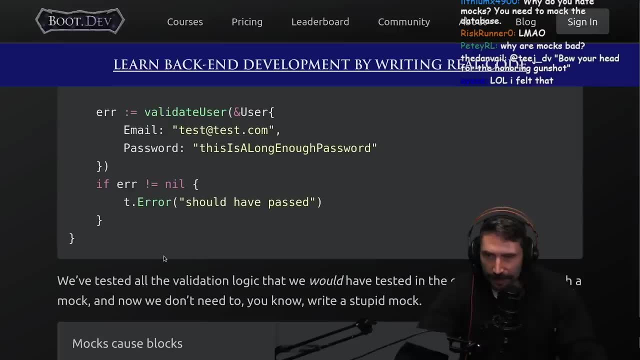 But what if you break it down? What should we call then Units? Yeah, The classic. your code is ass problem. Classic, really. Now we have to write a neat little test Test user: Yep, Bap, bap, bap, bap, bap. 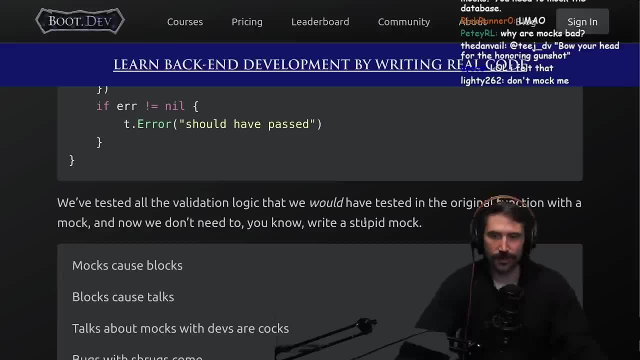 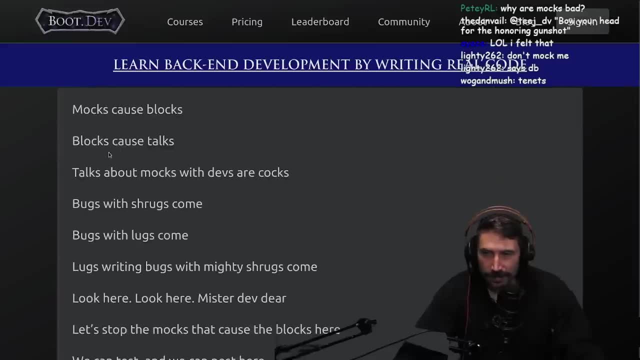 Awesome, We've. we've tested all the validation logic we would have tested in the original function with a mock And now we don't need to, you know, write a stupid mock, Absolutely. Mocks cause blocks, Blocks cause talks. Talks about mocks with devs are cocks. 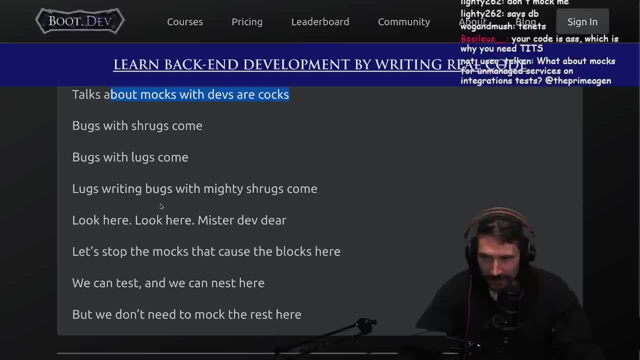 What Bugs with shrugs come. Bugs with lugs come. Lugs with bugs with mighty shrugs come. Look here. Look here, Mr Dev dear, let's stop the mocks that cause the blocks here. We can test and we can nest here, but we don't need to mock the rest here. 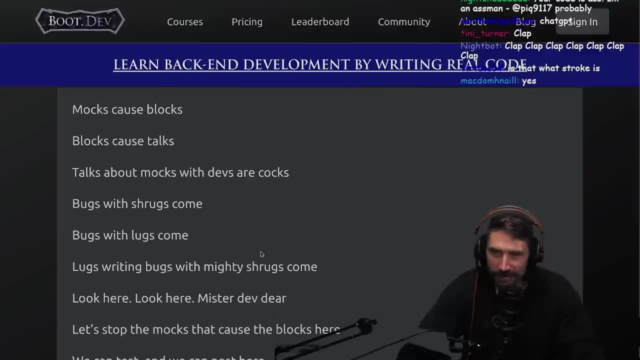 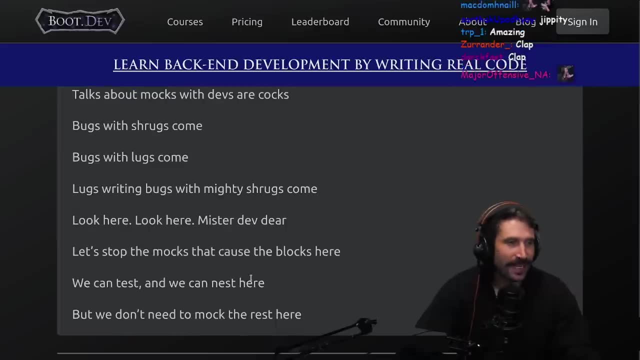 Probably chat jippity, but the Dr Seuss is beautiful. Okay, Mocking is akin to reading. Dr Seuss, Your mouth does a bunch of movements that your brain can't quite understand at all. This was most excellent. I love this. 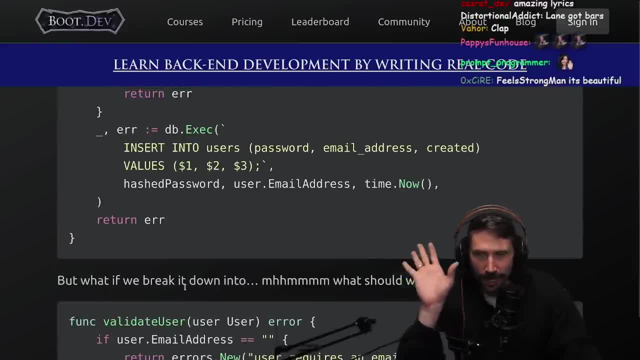 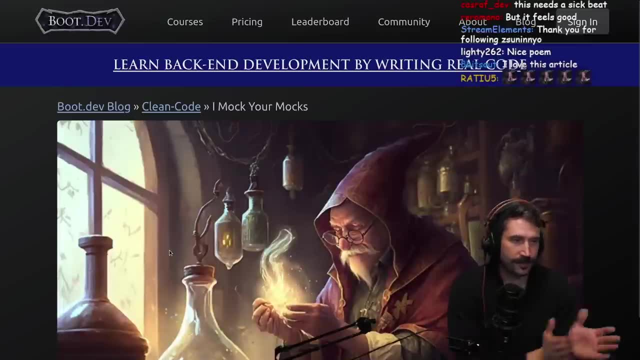 I'm full on this team. by the way, This is a full on team. Stop mocking. Write better back end code. Separate out your logic. Can we all give a little claps for Lane? This was a great article. Again, this was sponsored, but still I actually really liked the article. 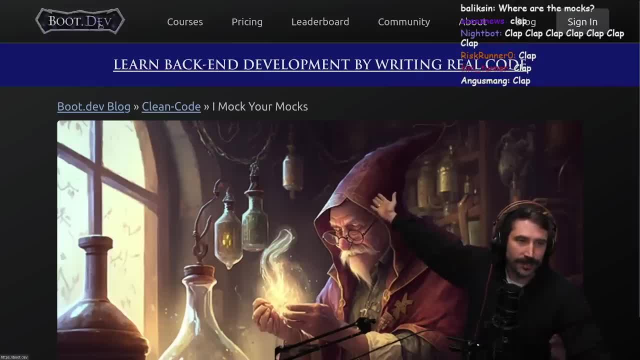 Check out boot Dev, boot Dev, helping your back end journey. Okay, And Lane's- actually he's an awesome engineer. I would not promote this if I thought Lane was a dummy. He's not a dummy. He's significantly better than me at back end engineering.